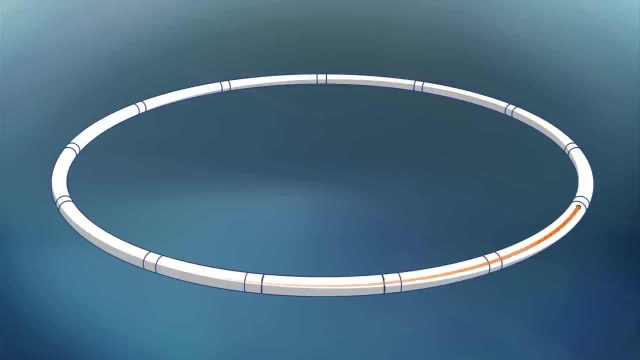 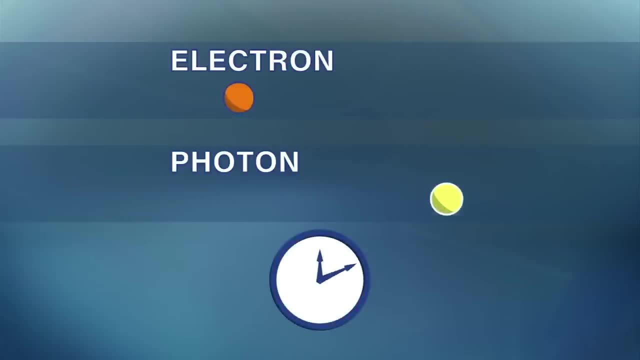 A previous accelerator sitting in the LHC tunnel holds the world record for velocity, accelerating an electron to a speed so fast that if it were to race a photon of light it would take about 14 minutes for the photon to get a lead of about 10 feet. If that doesn't. 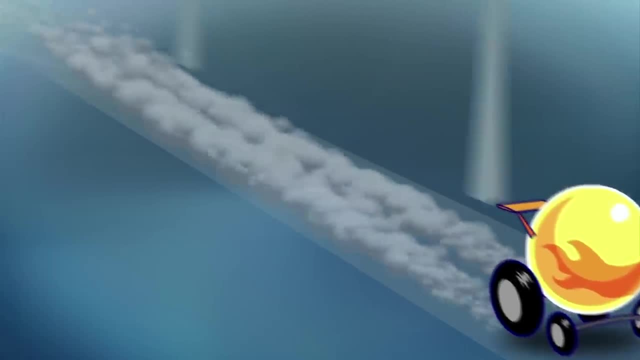 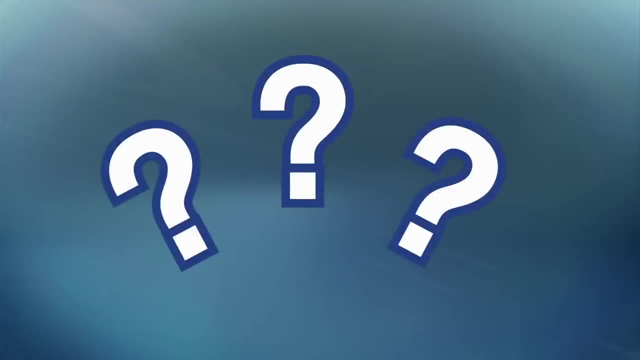 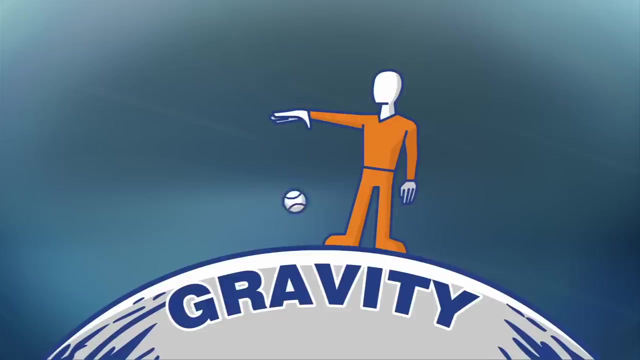 impress you remember, the photon is the fastest thing in the universe. It goes about 186,000 miles per second. So how do these subatomic particle accelerators work? Well, they use electric fields. Electric fields make charged particles move in the same way that gravity will pull a drop baseball. 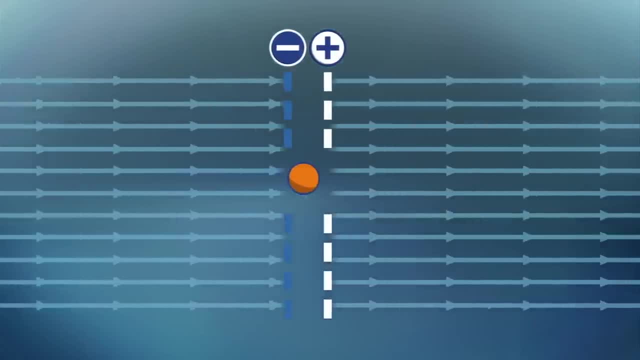 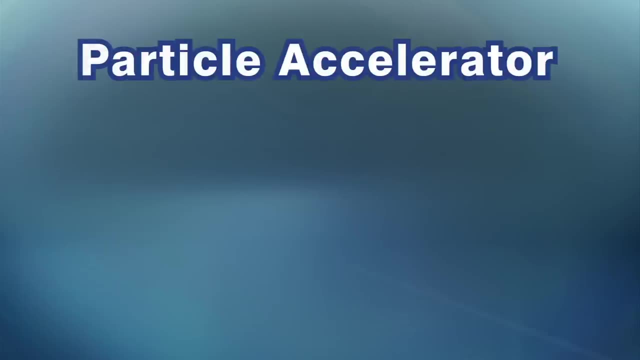 The force from the electric field will pull a particle and make it move. The speed will continue to increase until the charged particle is moving incredibly fast. A simple particle accelerator can be made by hooking a particle with a hook. If you have a hook, you can hook a particle. 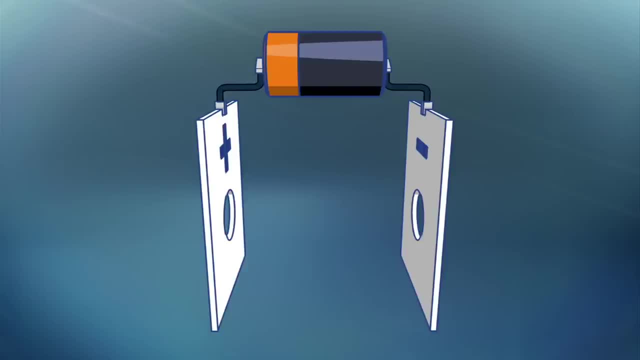 using two parallel metal plates to a battery. The charge from the battery moves onto the two metal plates and makes an electric field that pulls the particle along, And that's it: You've got a particle accelerator. The problem is that an accelerator built this way is very weak. 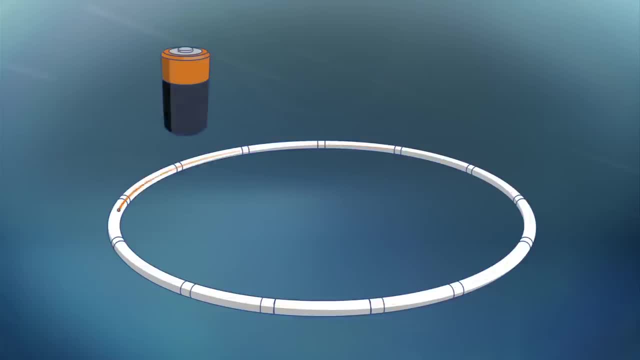 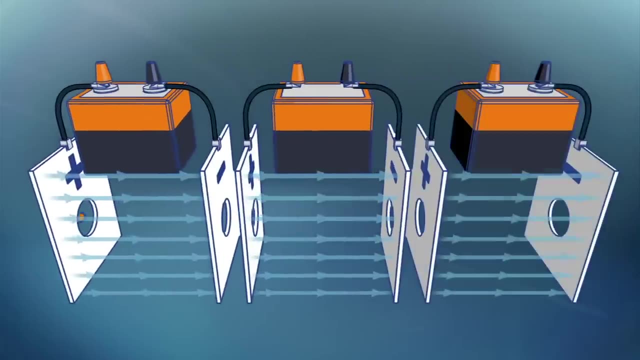 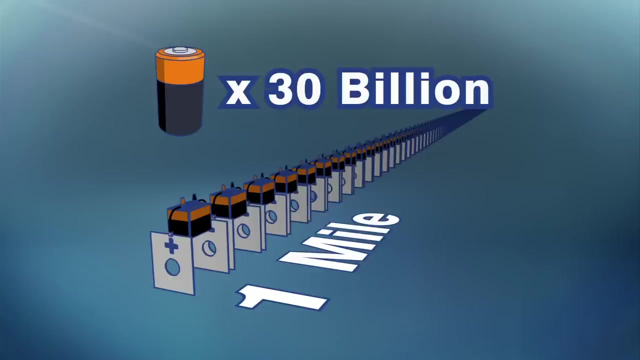 Building a modern accelerator like the LHC this way would take over 5 trillion standard D-cell batteries. So scientists use much stronger batteries and put them one after another. An earlier accelerator used this method and was about a mile long. It was equivalent to about 30 billion batteries. However, to make an accelerator, that is equivalent. 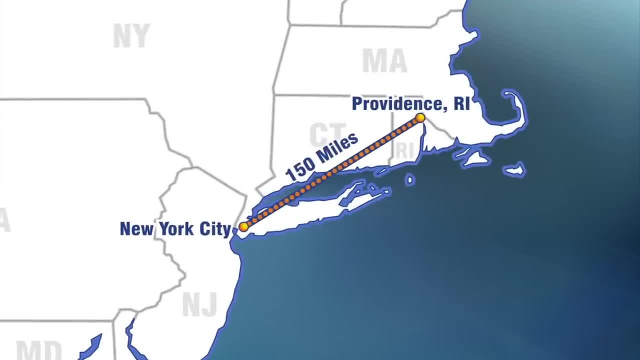 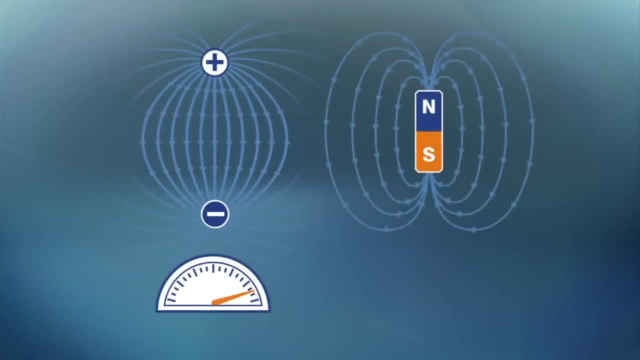 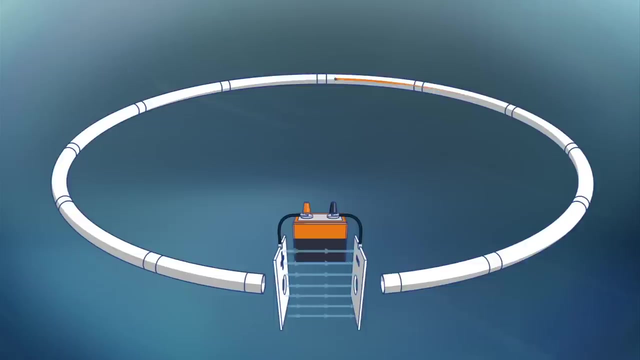 to 5 trillion batteries would require an accelerator 150 miles long. Scientists needed another way. While electric fields will make a particle go faster, magnetic fields make them move in a circular path. If you put an electric field along the circle, you don't need to use miles of. 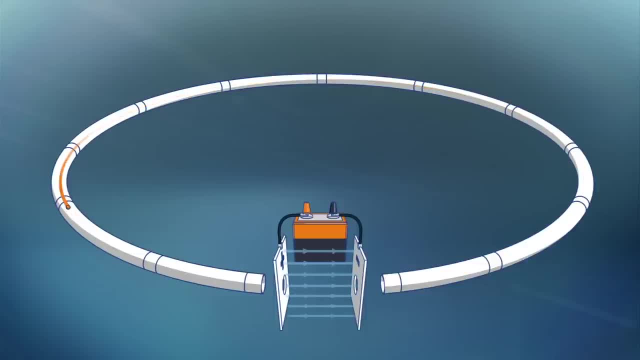 electric fields. You can use a single electric field over and over again. The beams go around the circle and each time they gain more energy. So very high energy accelerators consist of a short region with accelerating electric fields combined with a long series of magnets that guide the particles in a circle. The strength of the 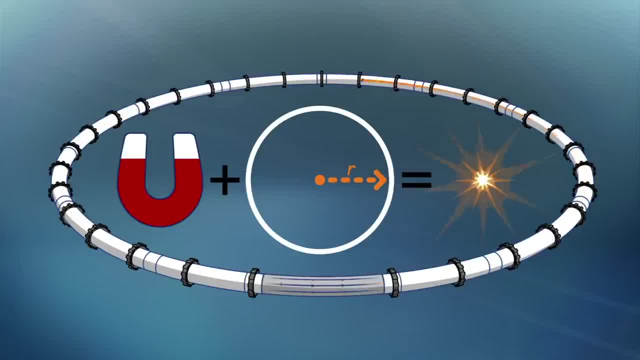 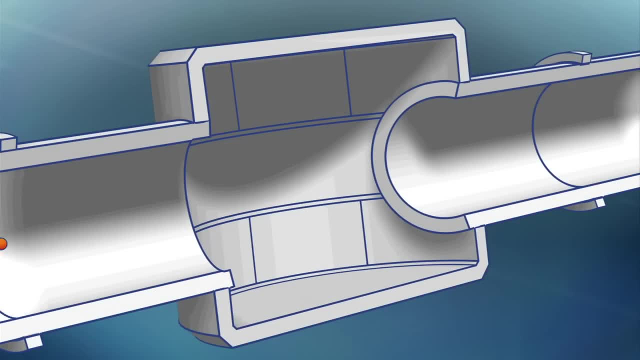 magnets, and the radius of the circular path determines the maximum energy of the beam. Once the beam is zooming along, then the real fun begins: The smashing. The reason physicists want to get those particles moving so fast is so they can slam them into one.